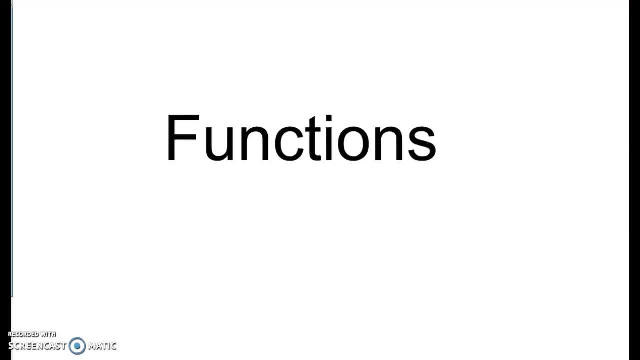 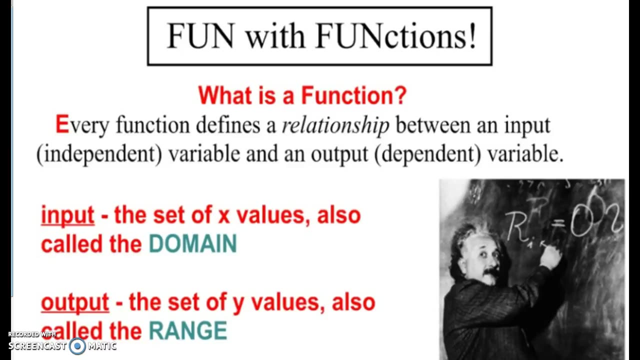 Today I'm going to go through a few problems with functions, with input and output, whether you're given the x value or whether you're given the y value, the range or the domain. we're going to talk about all those things Now. we had these in our notes, but what is a function? A function defines a relationship between an independent variable and a dependent variable, like our input and output, our x and our y. 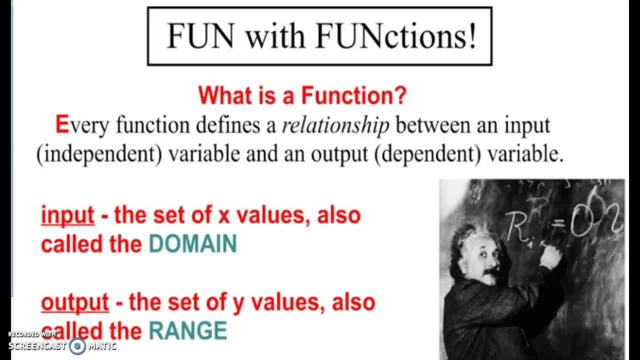 So if you don't have these inputs and outputs in your notes, pause the video, take a minute and write them down. Input is the x values- we also call that domain- and output is the y values, and we call that the range. 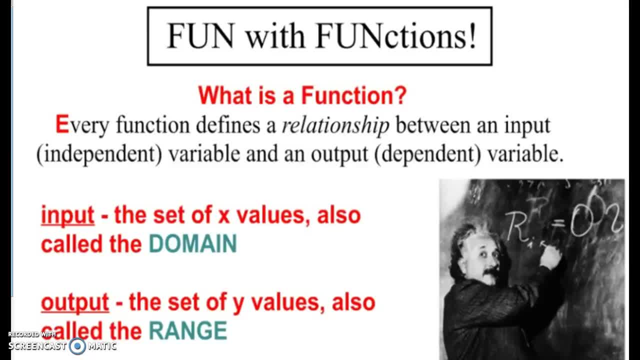 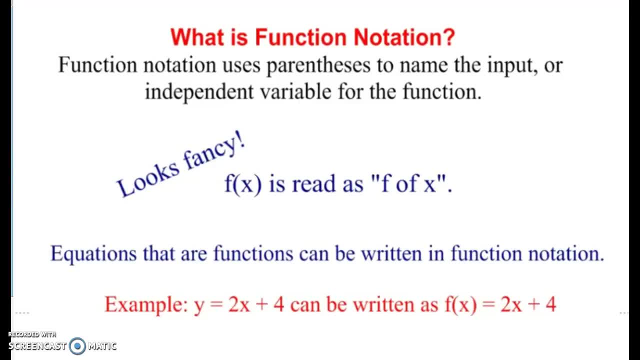 So a couple different words we're going to throw around with x and y. And what is function notation? I like to think about it as just a fancy way of writing a linear expression, Writing equations. Instead of writing our y equals, we end up for a function. we just write it as f of x equals. 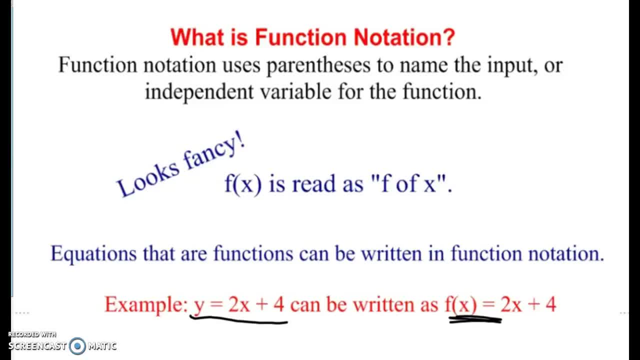 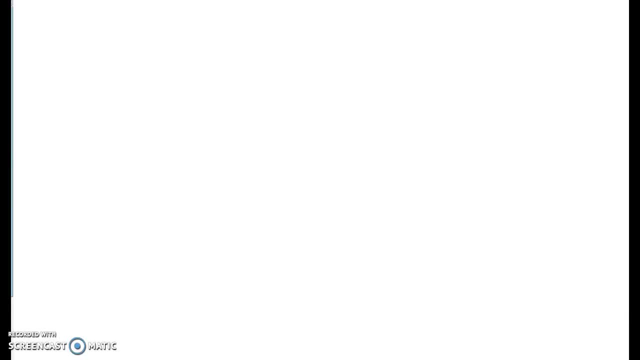 And that f of x. that stands for a function. Let's go through a couple of problems. Let's start with an easy function. We'll say f of x equals 2x plus Plus three. And let's say we are given f of four. 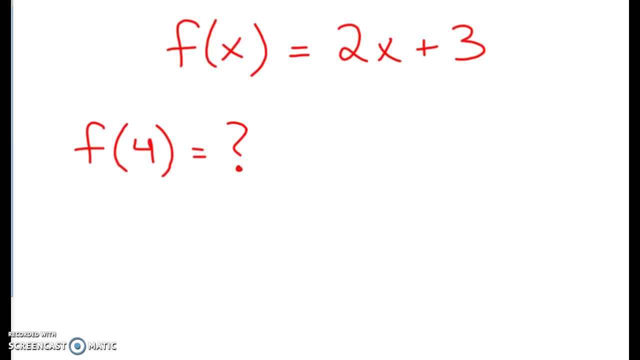 And they want you to know what that equals. What is f of four Now, when it's shown like this: notice that the four is in place of the x value. So that means we're going to plug four in where x is in our function and solve. 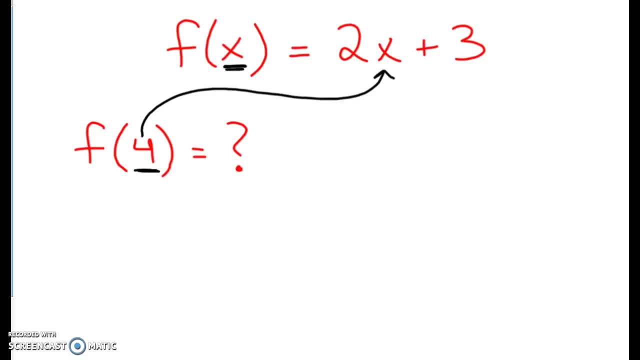 Because four is x, the place where x is. so we're gonna write it out: okay: f of x equals two times four. we're replacing that x with the four and then we just solve: okay, orders of operations. two times four, we get eight plus three, okay, so f of x now equals eight plus three, which we know is 11. okay, so now we can say: 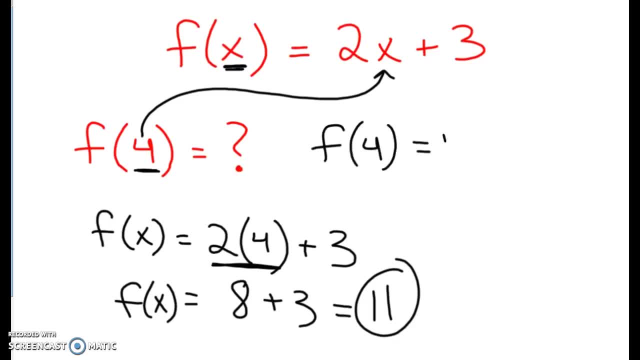 f of 4 equals 11. okay, and for that was an input right, because we were given the x value. okay, and 11 would be our output value. okay, let's go through a few more. let's say we were given f of x equals 8 plus 3. okay, so f of x equals 8 plus 3 equals 11. okay, so f of x equals 8 plus 3. 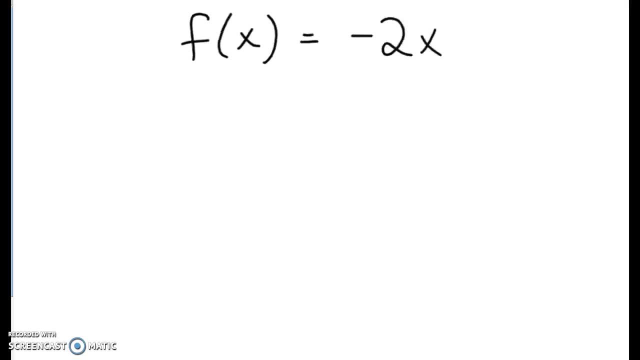 x equals negative 2x minus 7.. And let's say we have f of negative 4 this time, And they want to know what that is. Now, again, we were given our input value, or our x value. Notice that negative 4 is in place of where the x usually goes in our function. So we're going to plug negative 4. 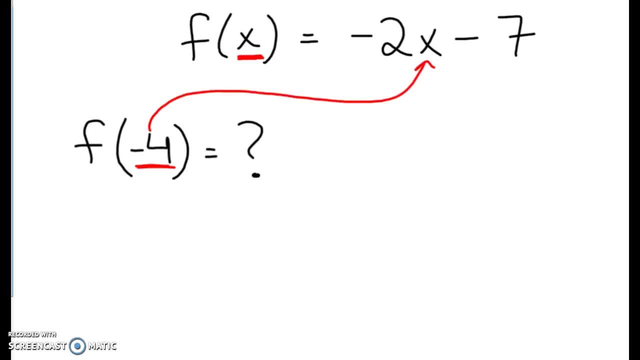 in for x in our function. So we have negative 2 times a negative, 4 minus 7.. Orders of operations: we do our multiplying first. So negative 2 times a negative, 4. A negative times a negative is always a positive, If you need to check that in your calculator. 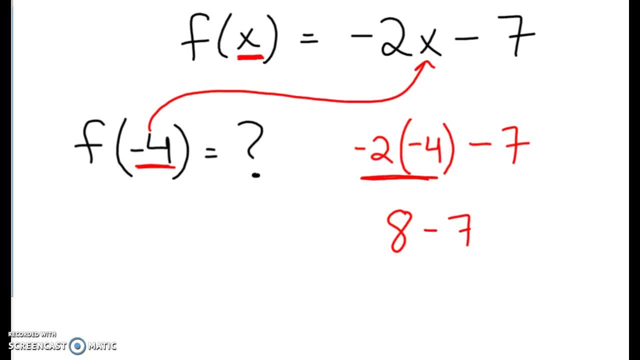 make sure you're doing so. And then we still have minus 7.. And 8 minus 7, we get a positive one, okay. so f of negative four equals one, okay. so now let's say we have a new function: f of x equals. 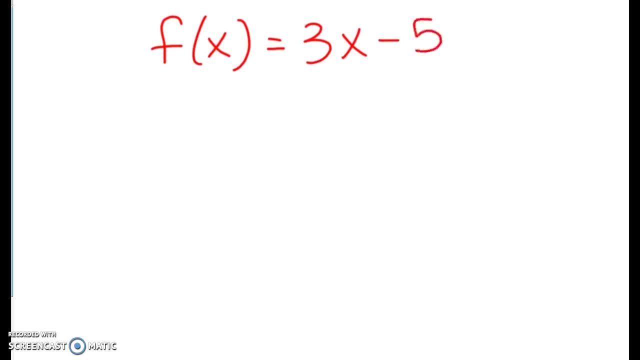 three x minus five. okay, and this time let's say we, instead of given an input value, let's say we were given an output value. okay, so let's say we were given an input value of of 10.. okay, so let's say we are given 10 here. 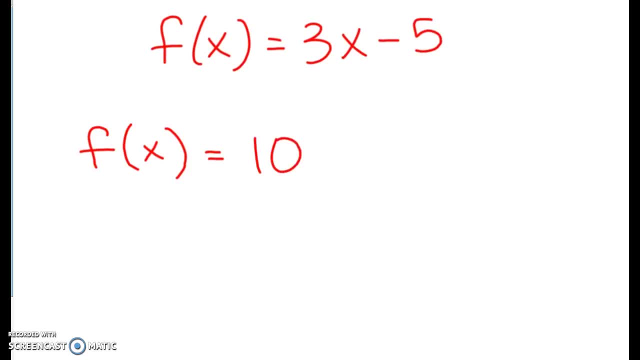 and now notice that 10 is not in the place of x, so that means it's something different. okay, we're not given our input value anymore. now we're given our output value. so notice how this looks different than if our 10 was inside our parentheses. 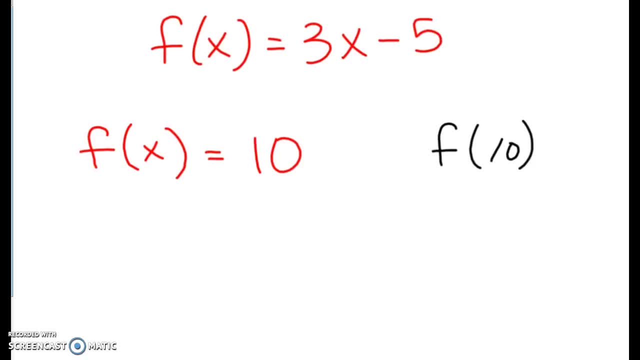 okay, Now we have to set this up a little different. then Now notice it says f of x equals 10.. Well, notice we have an f of x here. So can't I just replace that whole f of x with 10?? 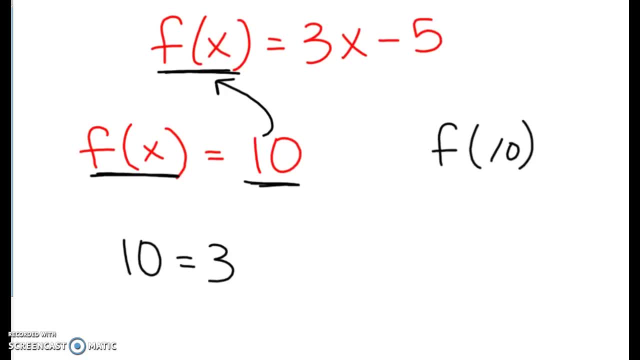 So now I'm going to set it up as 10 equals 3x minus 5.. Because I'm trying to find that input value. I'm trying to find that x value now. Okay, now, with multiple step equations, we are going to solve for x. 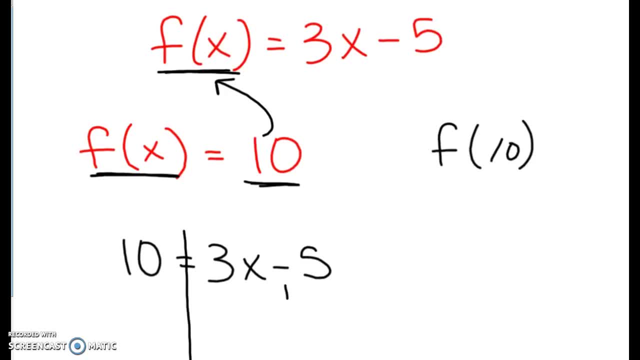 So we draw our line down. First, we're going to add 5. So we get 15 equals 3x, 15 equals 3x, And next, our final step, we're going to divide by 3.. Okay, so I'm just going to rewrite my work up here. 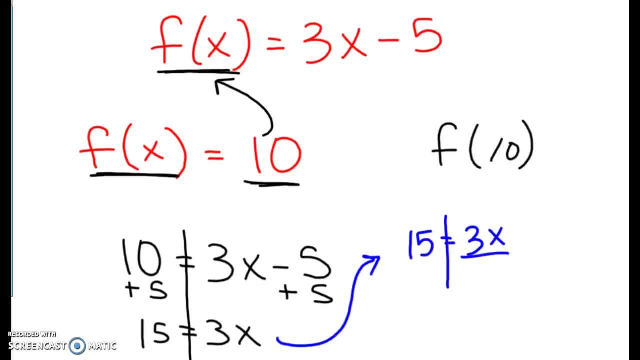 So we had 15 equals 3x. Okay, and we divide by 3.. So we get x equals 5.. Okay, so now we know that our input value is going to be 5 for this function when we're given the output value of 10.. 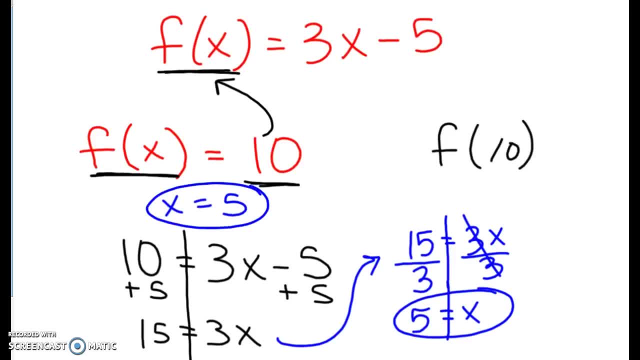 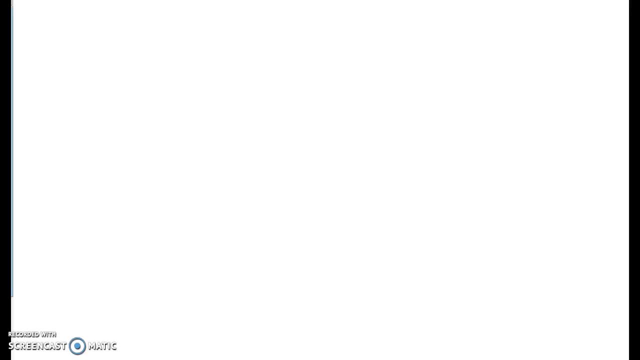 Okay, so now we know x equals 5.. All right, let's do one more where we're given an input, An output value and an output value, and we'll set it up for each one. So let's say f of x, our function equals negative 3x plus 7 for this one. 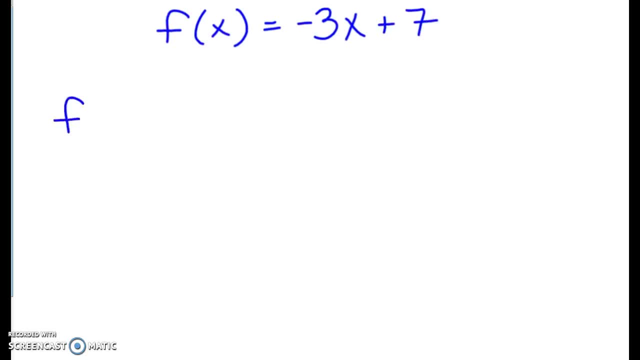 Okay, now for this time. let's say we're given f of 2.. Okay, and we want to know what f of 2 equals. And our other problem. let's say we want to know what f of x equals when we have 16 as our output. 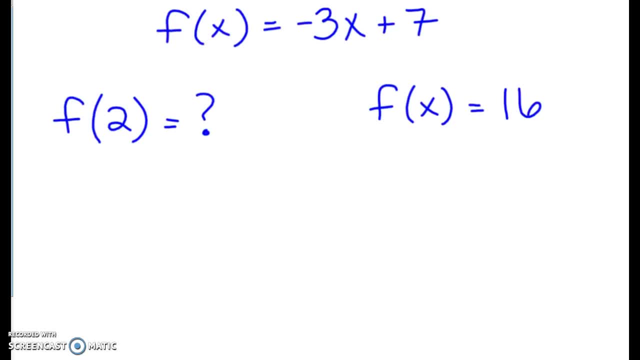 Okay, so we have two different problems with the same function. Okay, so they're set up a little differently, Okay, because remember our first one. Okay, our 2 is in the place of where x is, So that means we're going to plug in 2 for x. 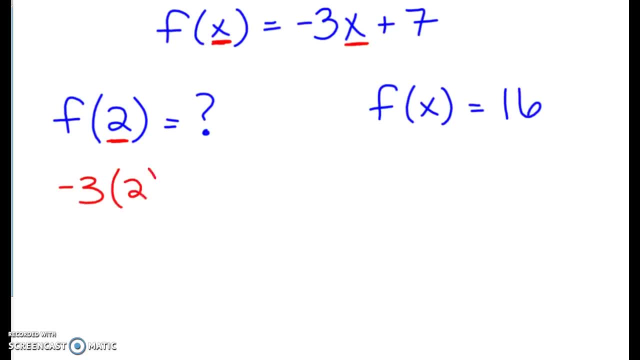 Okay, so we get negative 3x. Negative 3 times 2 plus 7.. Okay, and we just solve that with orders of operations. Negative 3 times 2, we get negative 6 plus 7.. Negative 6 plus 7 is just 1.. 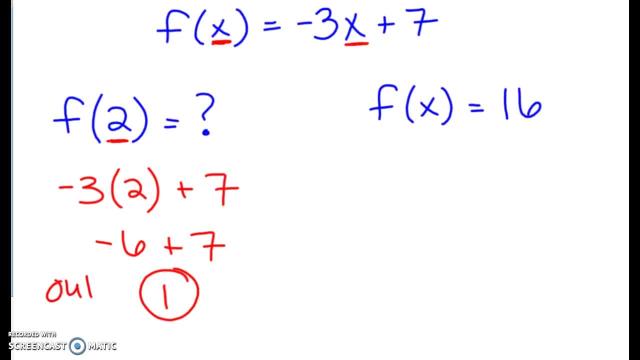 Okay, so 1 would be our output value when our input value is 2.. Okay now, this time we are given an output. Okay, so we need to find the input value. Okay, now notice how it's set up- a little different. 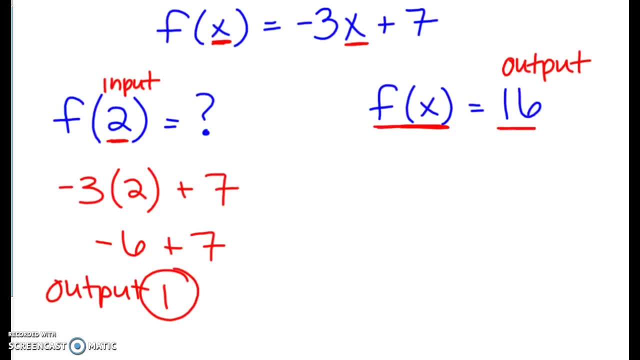 how it says f of x equals 16.. Okay, so when f of x equals 16, okay, we're going to plug in 16 for this entire f of x. So we're going to set up a multiple step equation. So we get: 16 equals our function, negative 3x plus 7.. 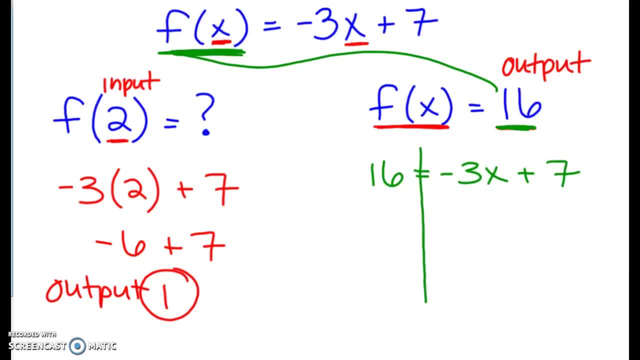 Okay, and we draw our line down if that's helpful. Okay, and we're going to subtract first. We always add or subtract first when we're doing two-step or multiple-step equations. Okay, so then we get 9 equals negative 3x. 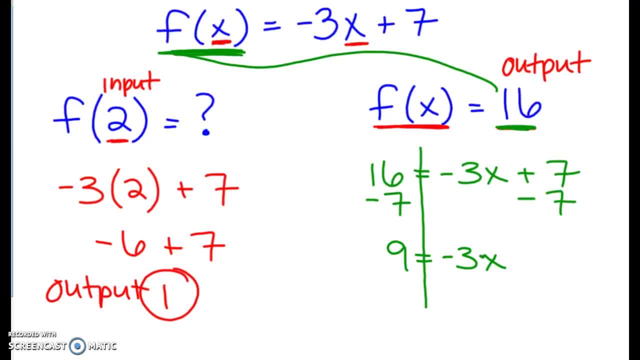 Then our final step: since there's multiplication going on between the negative 3 and x, we're going to divide by negative 3.. Divide by negative 3.. And we get x to equal negative 3.. Okay, so that was our input value. 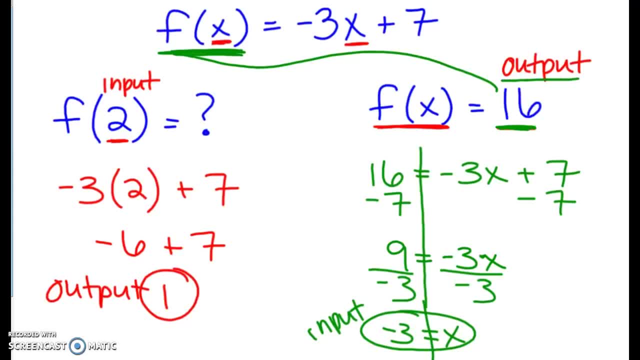 okay when we were given an output of 16.. So notice how these two problems are set up a little differently. Okay, we have the same function. okay, but one we were given the input and another we were given the output. 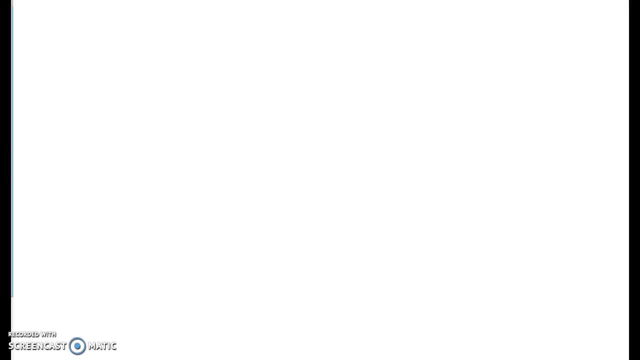 All right, let's try this. Try one more: f of x equals 4x minus 6.. Okay, let's say we were given f of 5.. Okay, and we want to know what f of 5 equals. And let's say we have f of x equals 10..